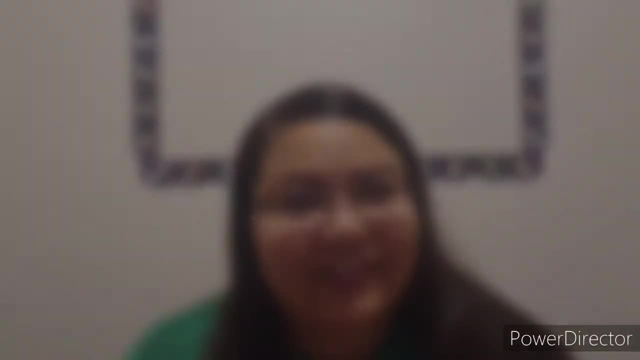 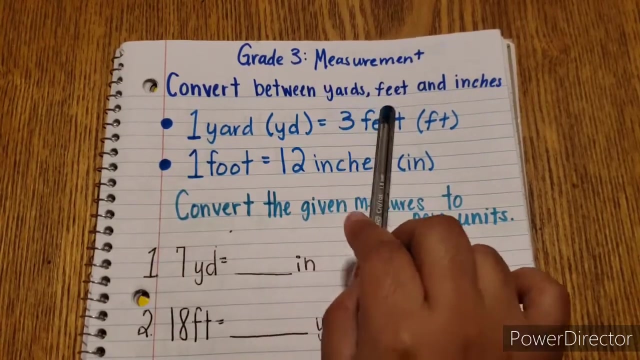 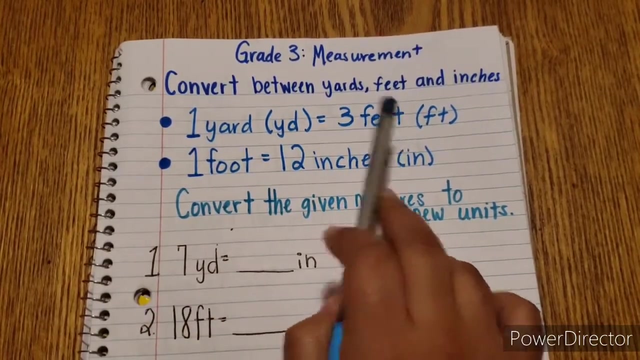 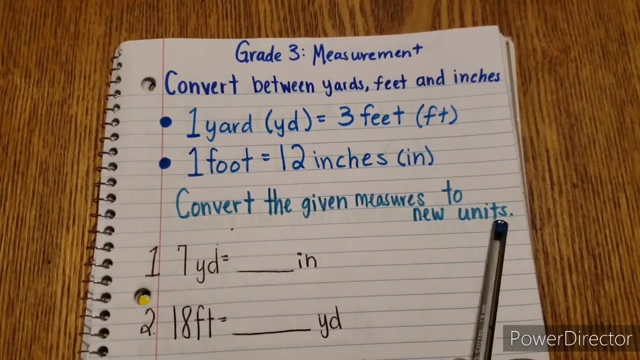 consist of what I'm about to go over. I hope you guys enjoy. Let's get started with grade 3 measurement. We are going to convert between yards, feet and inches. So here I have 1 yard equals 3 feet and 1 foot equals 12 inches. So we need to convert the given measures. 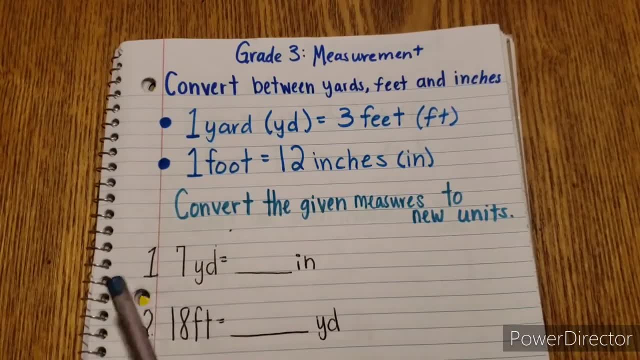 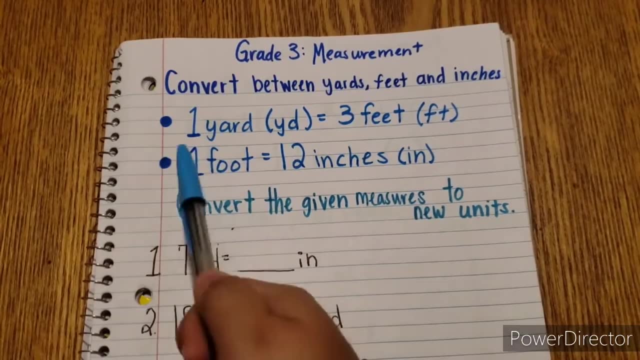 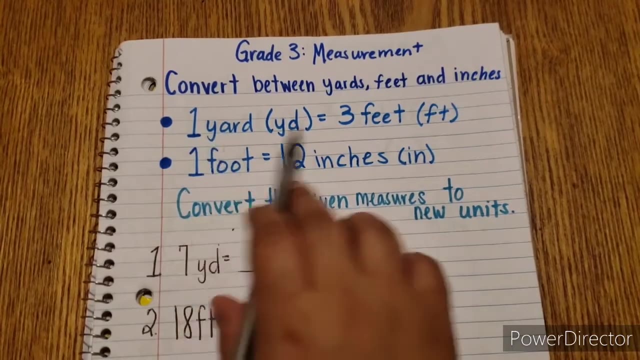 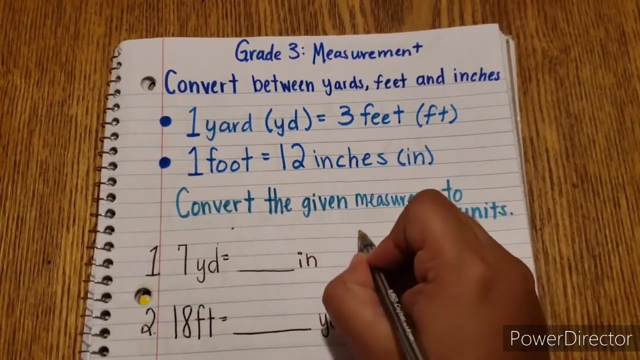 to new data units. so let's start with number one. we have seven yards and we want to get inches. so first we're going to go from yard to feet, from feet to inches, so let's go from yard to feet. so if one yard equals three feet, how many feet are there in seven yards? we would do seven times three and that is. 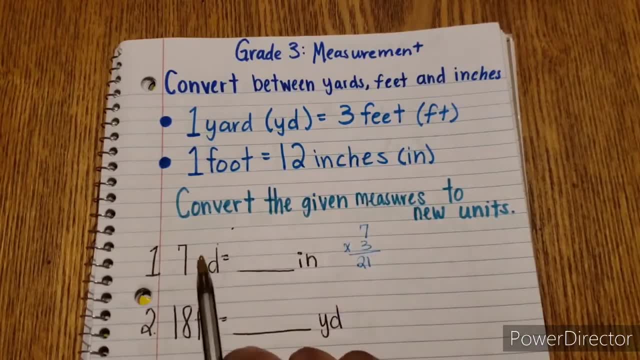 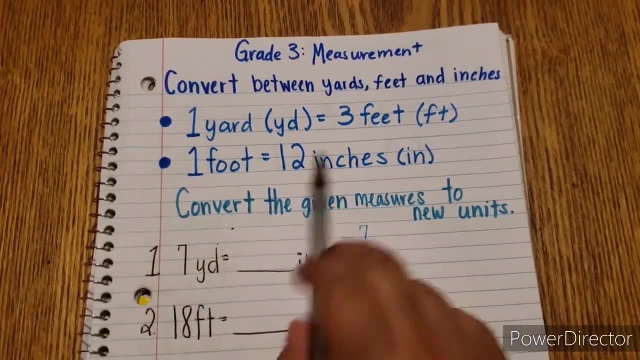 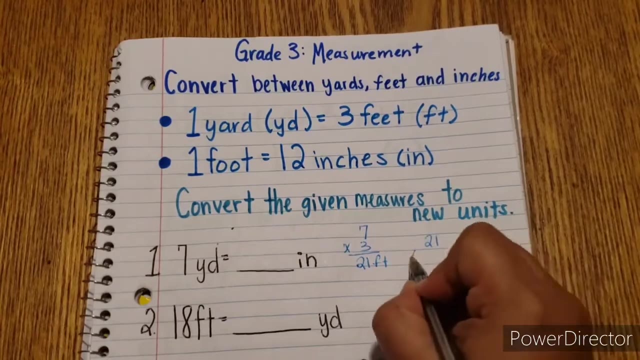 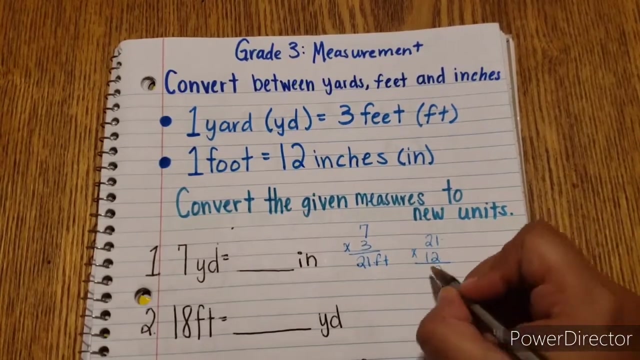 21. so there is 21 feet in yards. now let's go from feet to inches. so on one foot there's 12 inches. so what we want to do is 21 times 12. so first we have: 1 times 2, that's 2. 2 times 2, that's 4. then we have 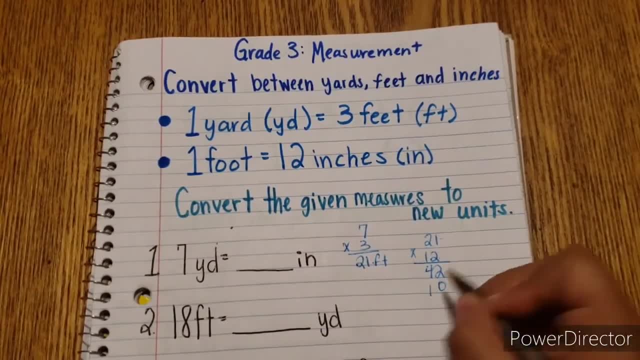 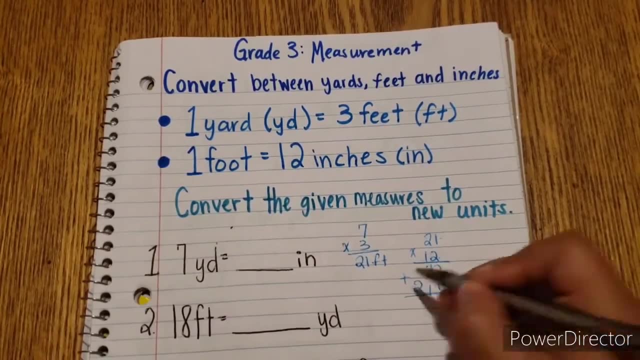 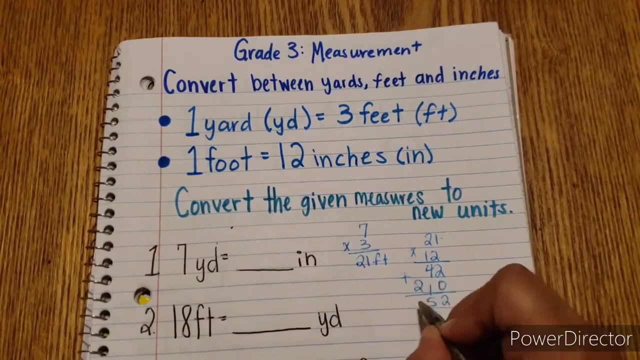 a 0, then we have 1 times 1, that is 1, and 2 times 1, that is 2, so we have 2 plus 0 is 2, 4 plus 1 is 5 and 0 plus 2 is 2. so this is 252 inches. 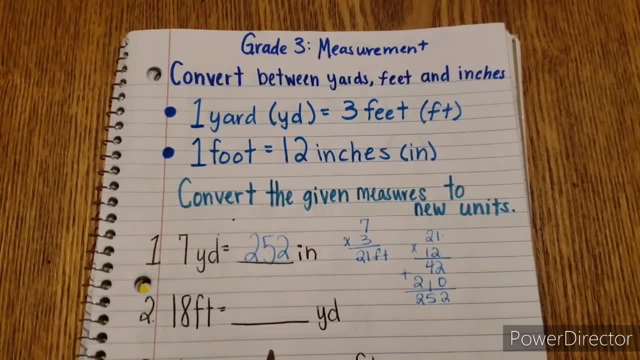 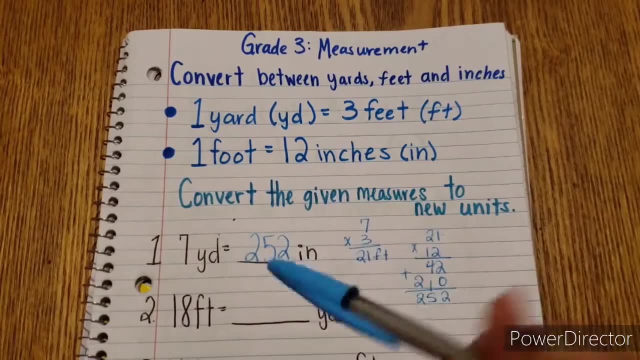 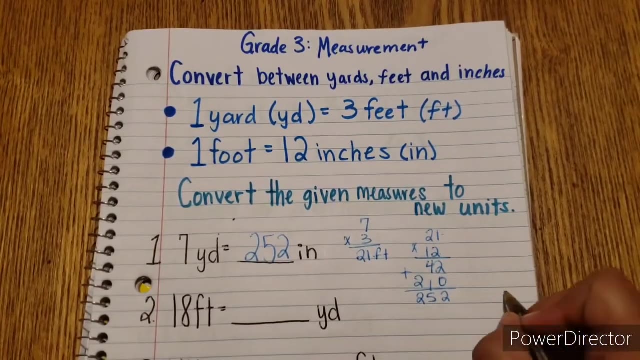 let's go on to the next one. we have 18. feet equals how many yards? so in one yard there are 3 feet. so now we have feet and we want to go into yards. so what we would do, we would get the 18 and we 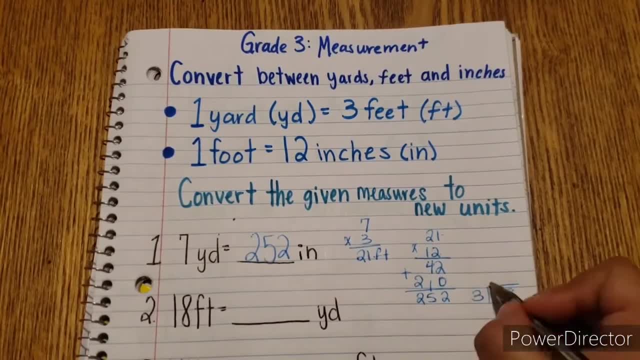 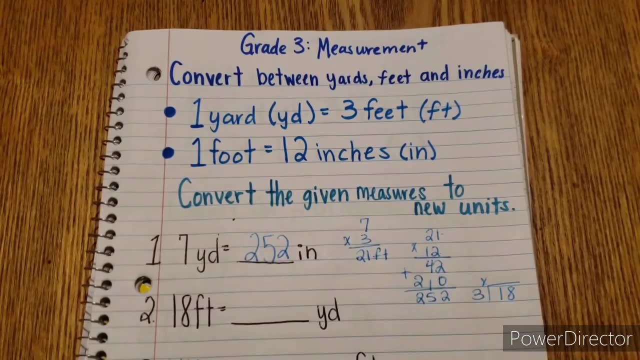 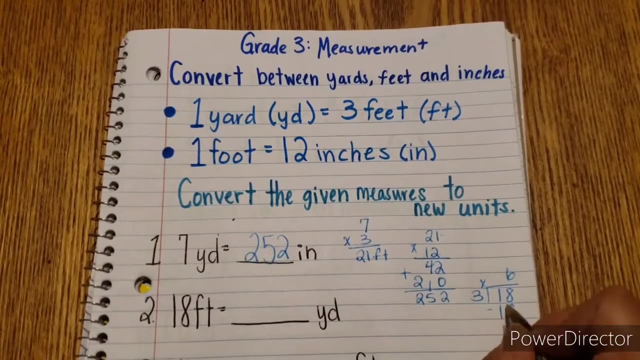 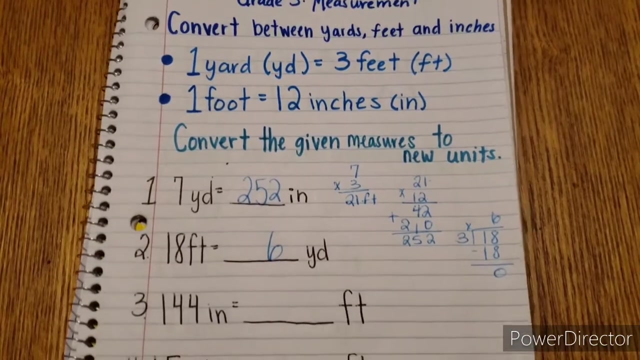 would divide that by 3 so we can figure out how many yards there is. so 3 times what equals 18. that would be 6. 3 times 6 equals 18. 18 minus 18 equals 0, so the answer is 6 yards. let's go on to. 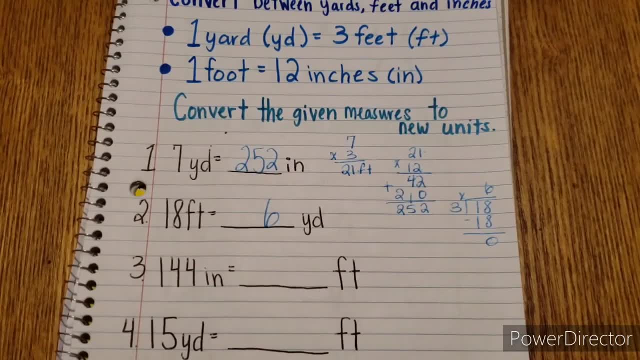 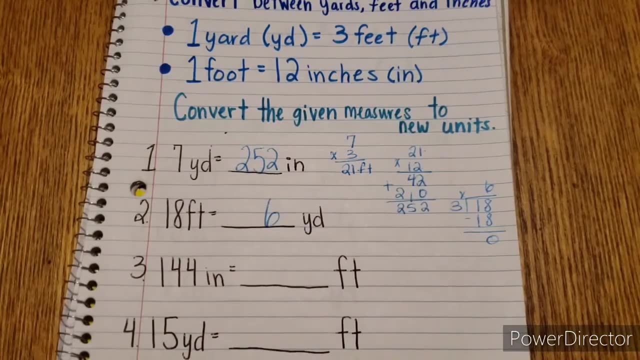 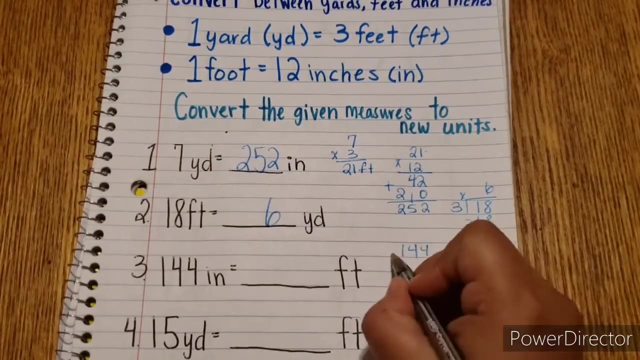 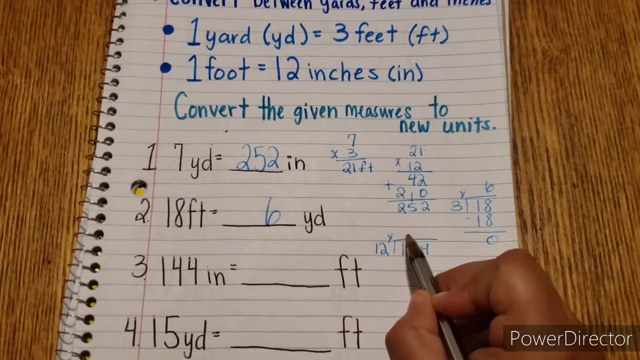 the next one. we have a hundred and forty four inches and we want to figure out the feet. so in one foot there are 12 inches. so the first thing we would do is a hundred and forty-four divided by 12, so we have 12 times what equals 1- nothing. so that's 0, 1 now. that's 0, 12 times. 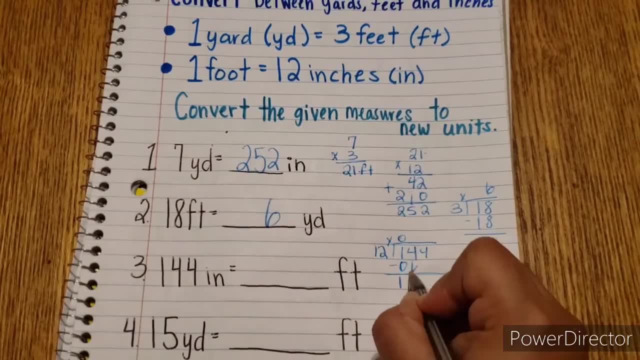 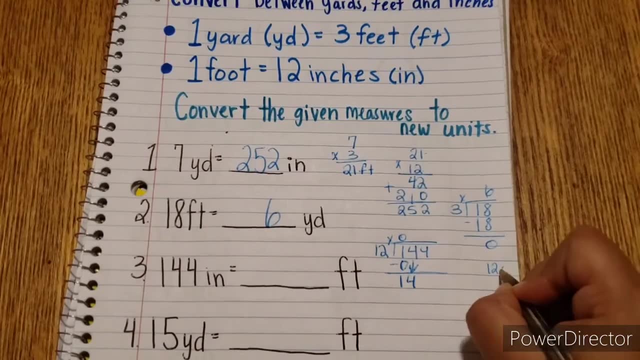 0 is 0, 1 minus 0, that's 1. we bring down the 4 12 times what equals 14. so let's go ahead and do that here. we have: 12 times 1 equals 12, 12 times 2 equals 15. so we have a hundred and forty four. 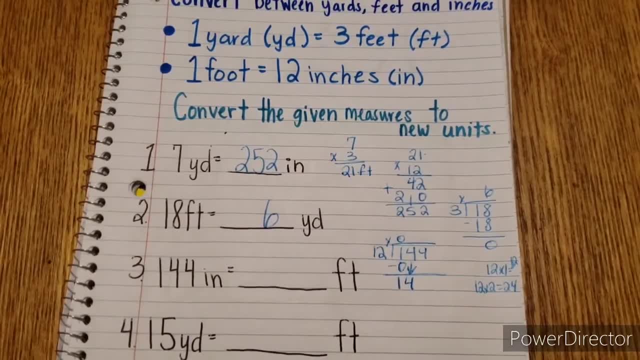 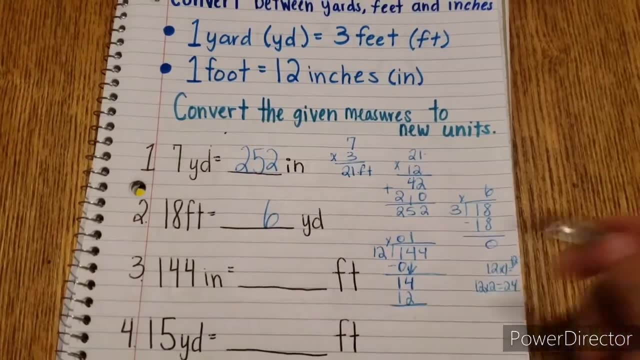 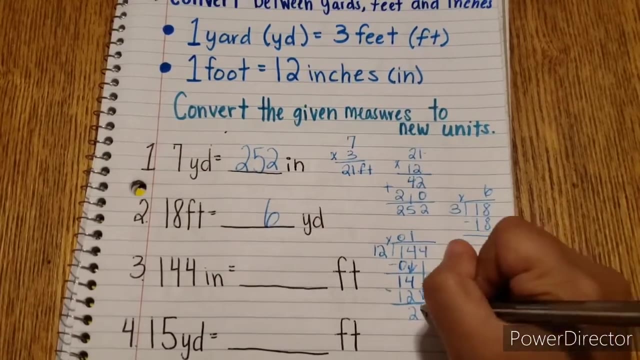 so we can see we don't have 14, but the closest would be 12. so we have: 12 times 1 equals 12. what is 14 minus 2, that is 2. we bring down the 4, now we have 24. so we have 12 times what equals 24. that 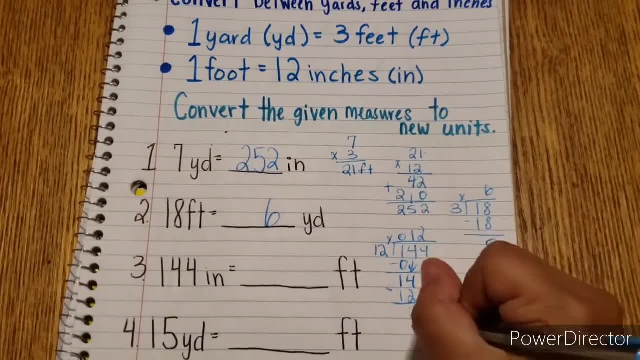 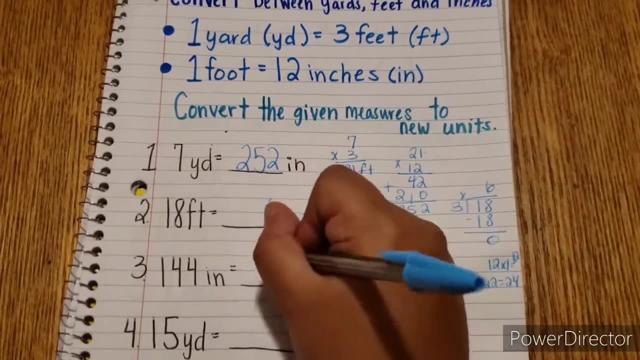 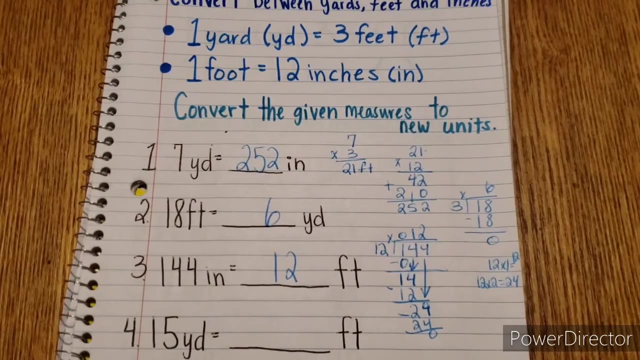 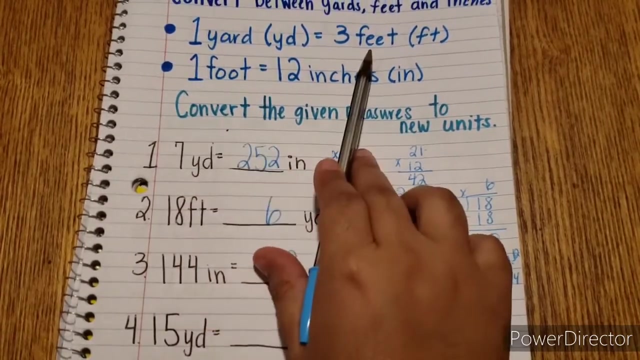 is 2, so 12 times 2 equals 24. you subtract that that is 0, so the answer would be 12. so 144 inches equals 12 feet. let's go on to the next one. we have 15 yards. equals how many feet? so 1 yard equals 3 feet. so if we have 15 yards, how many feet will? 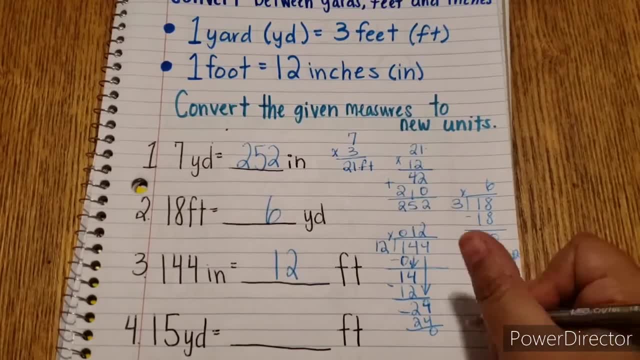 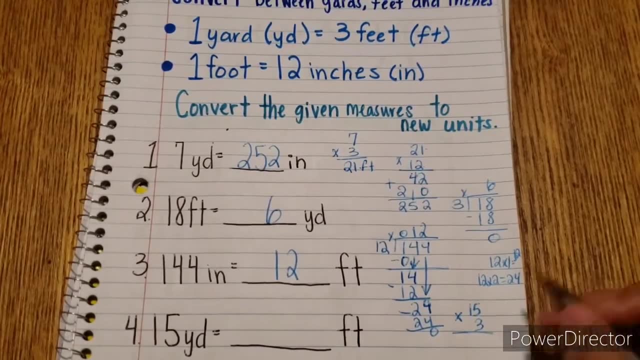 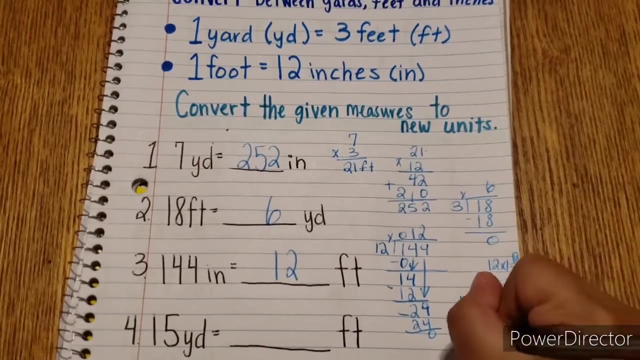 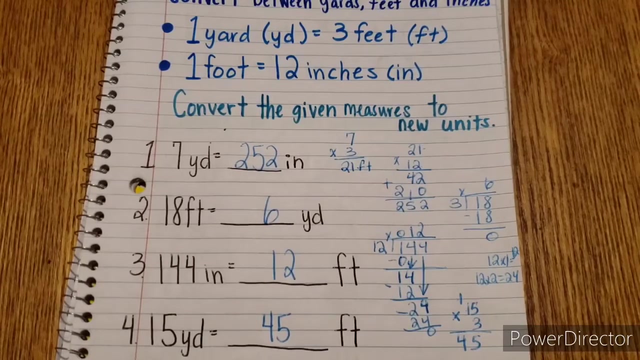 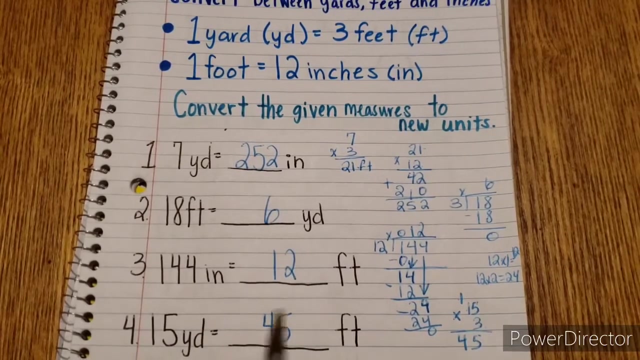 we have. what we would do is 15 times 3, so we have: 5 times 3 is 15. 3 times 1 is 3 plus 1 is 4, so that would be 45 feet. so if you're wondering why we're multiplying by 3, it's because we want to know yards. 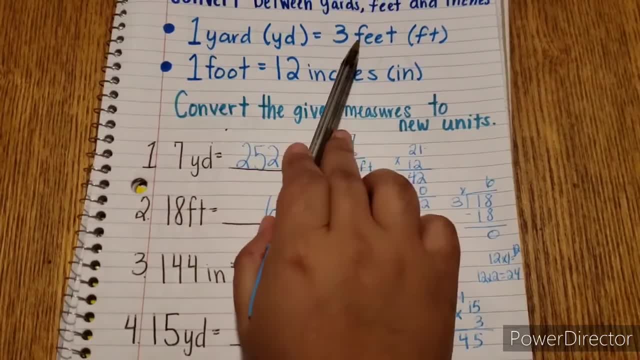 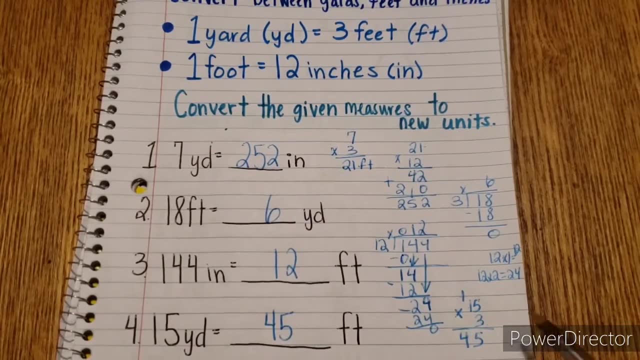 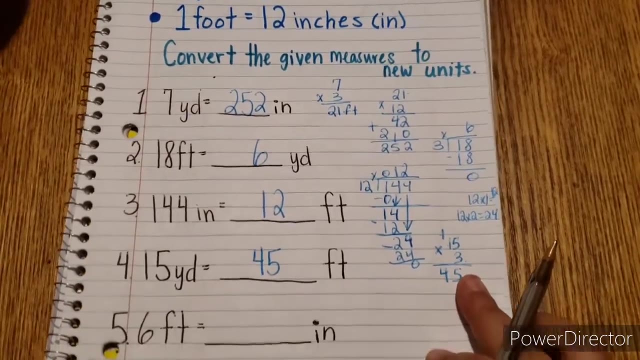 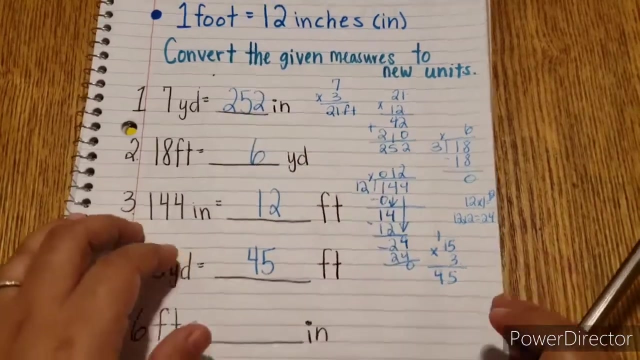 2 feet. so we have yards, 2 feet. 1 yard equals 3 feet, so how many feet would be in 15 yards? We would have to multiply 15 and 3.. So let's go on to the last one. We have 6 feet equals how many inches? So here we have: 1 foot equals 12 inches. So what we would do 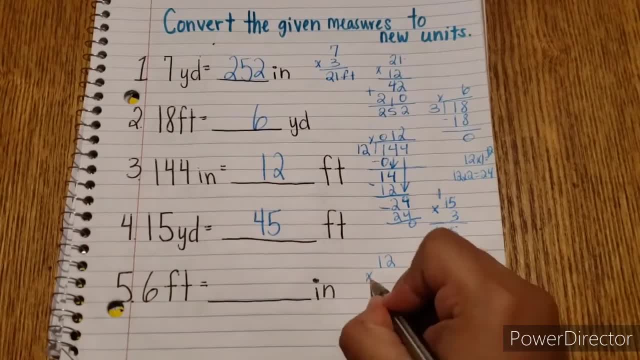 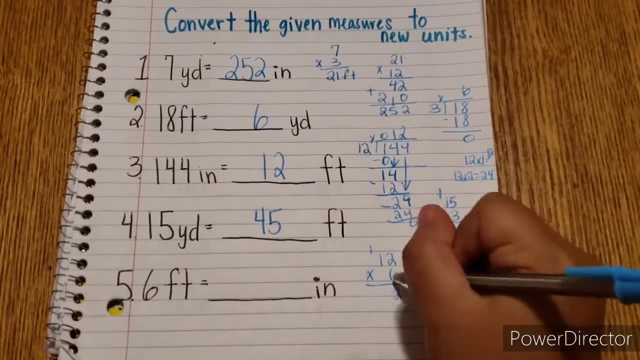 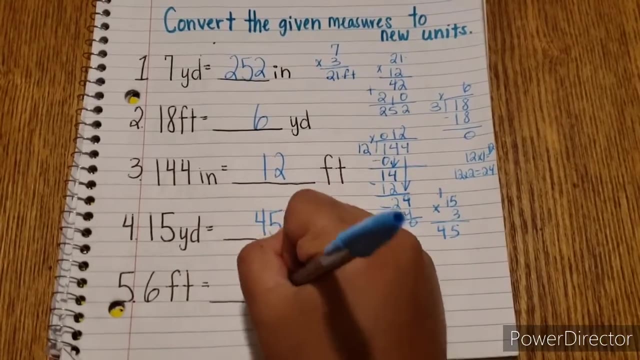 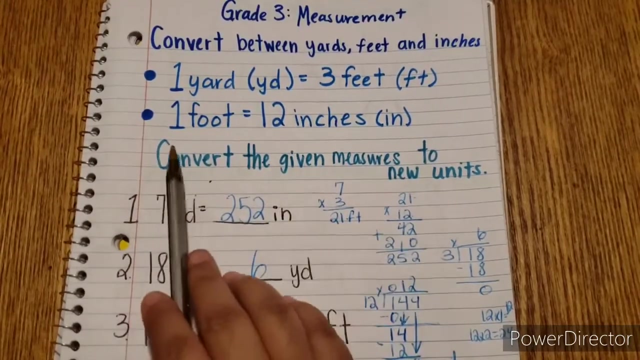 is 12 times 6.. So what is 6 times 2?? That is 12.. 6 times 1, that is 6 plus 1, that is 7.. So that is 72 inches. So again, 1 yard equals 3 feet and 1 foot equals 12 inches. Now we're going to get. 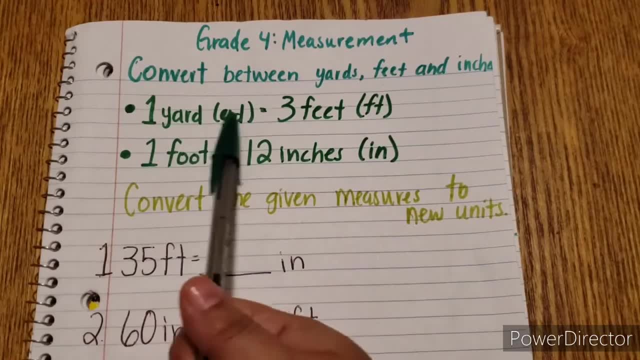 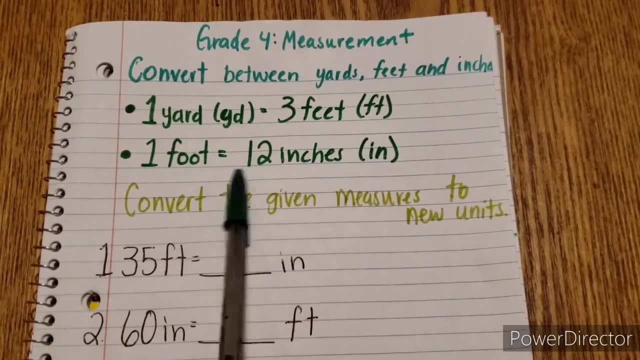 into grade 4.. In our measurement we need to convert between yards, feet and inches. So here we have: 1 yard equals 3 feet and 1 foot equals 12 inches. We need to convert the given measures to new units. 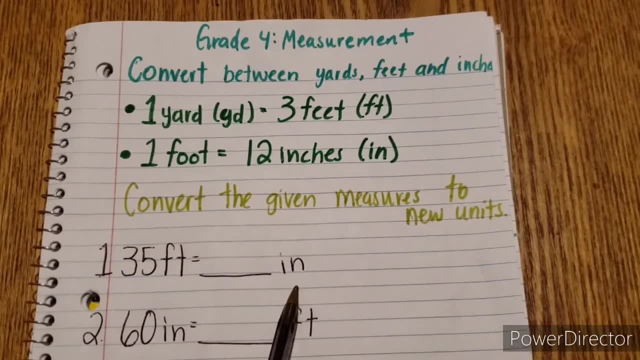 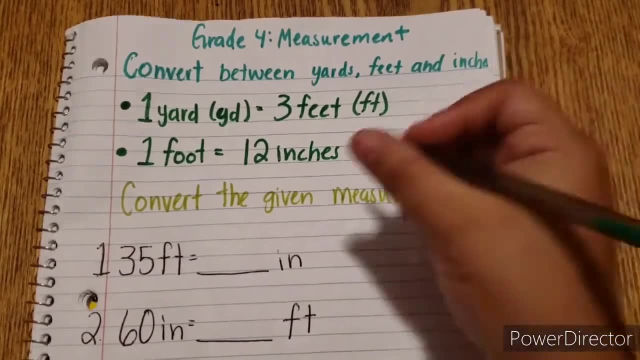 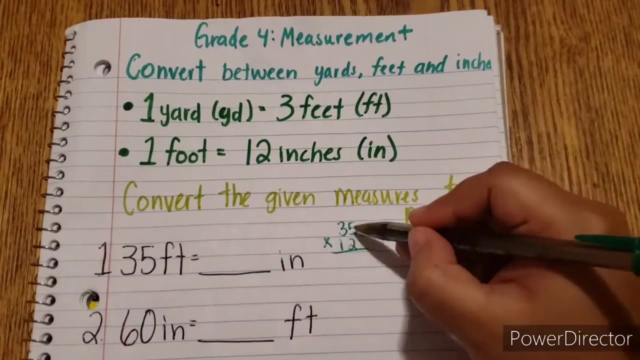 So here we have 35 feet. So how many inches are there in 35 feet? So on 1 foot there is 12 inches. So what we would need to do is 35 times 3.. 5 times 2, that's 6.. 3 times 6 equals 2.. 6 plus 1 equals 6.. Take a look here, in that bulge you caught. 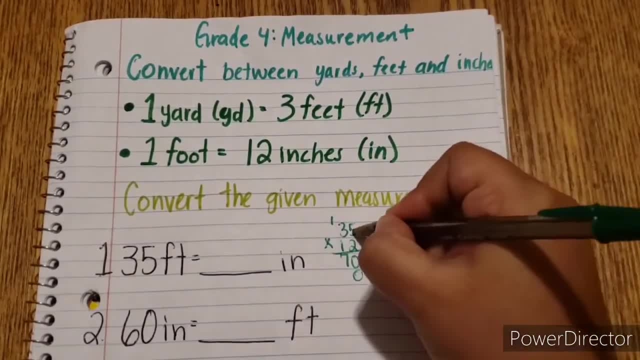 on this equation. Yes, that's 3 times 4.. 3 times 5 equals 3.. So what if the length of 4 is 10?? So that would be 27.. The length of 4 is 3.. If we go again to grade 2, and what we? 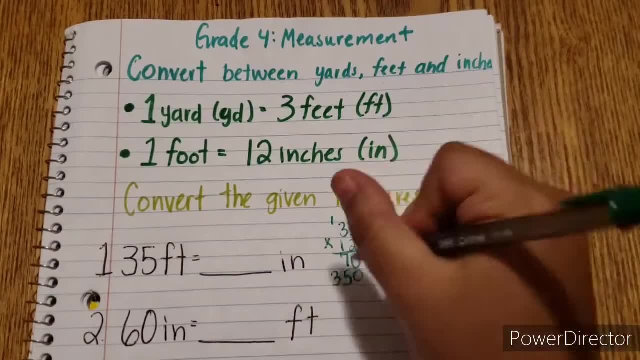 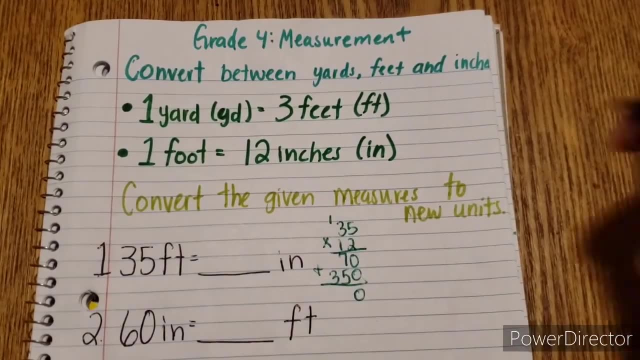 would do is 5 times 5 is 10 times 2.. Stop on that run, okay. How many inches does a wide yard need to be in order to convert between yards? so the width of 5 and 20 inches 35 times 5 equals 17, or 9 inches. So this is what we would need to express. So here we have 15 feet equals 3 feet and 12 inches. So here we have 17 feet equals 12.. 5 times 5 is 9 inches. So we would have: how many inches is that, raise始ling against 8 inches? 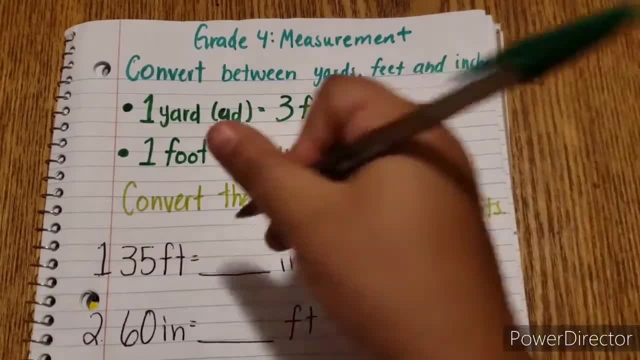 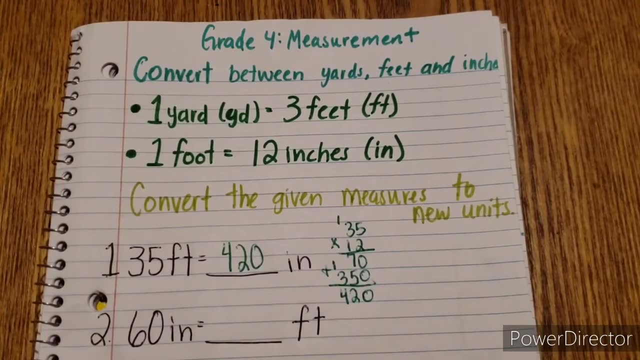 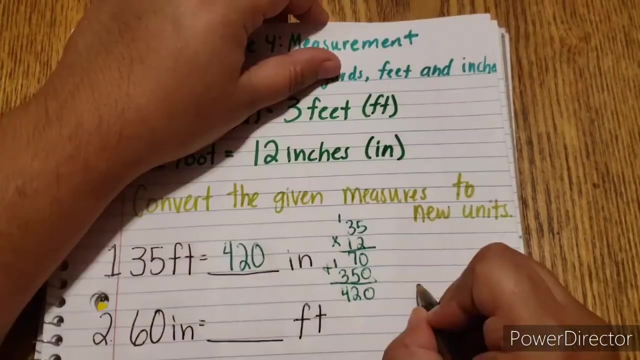 3 plus 1 is 4, so that is 420 inches. Let's go on to the next one. We have 60 inches and we want to go into feet, So what we're going to do is 60 divided by 12.. 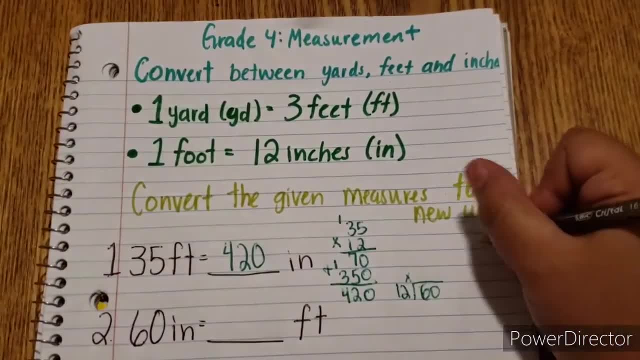 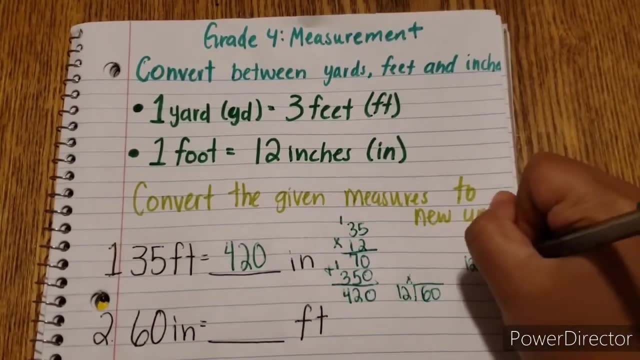 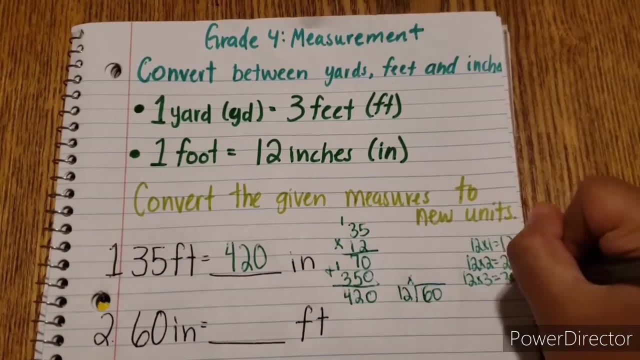 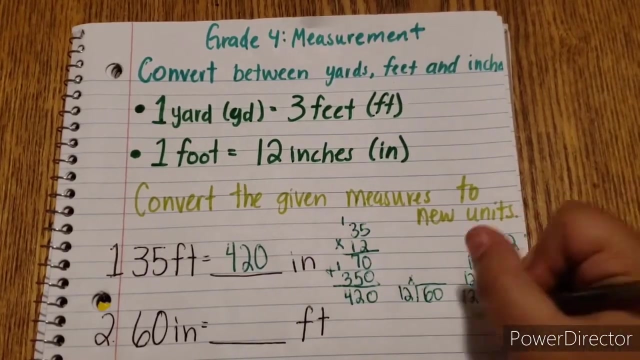 So here we need 12 times what equals 60.. So let's go ahead and do those here. 12 times 1 equals 12,. 12 times 2 equals 24,. 12 times 3 equals 36,. 12 times 4 equals 48,. 12 times 5 equals 60. 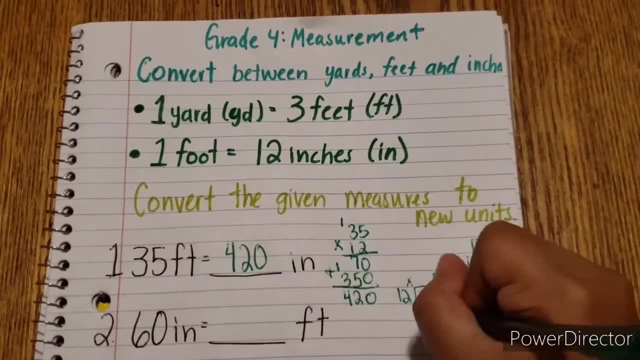 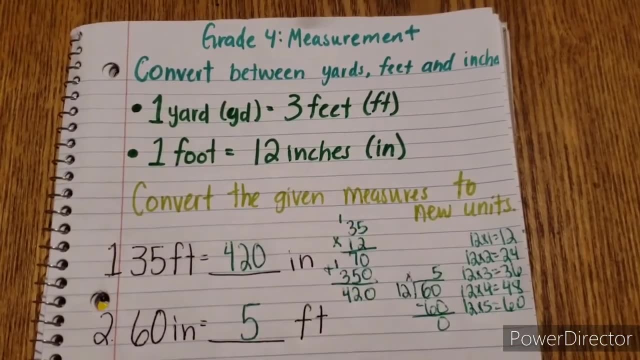 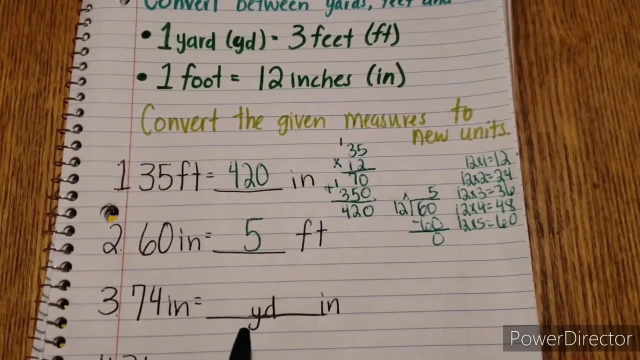 So 12 times 5 equals 60. Okay, 60 minus 60 is 0, so 60 inches equals 5 feet. Let's go on to the next one. We have 74 inches and we want to go into yards. 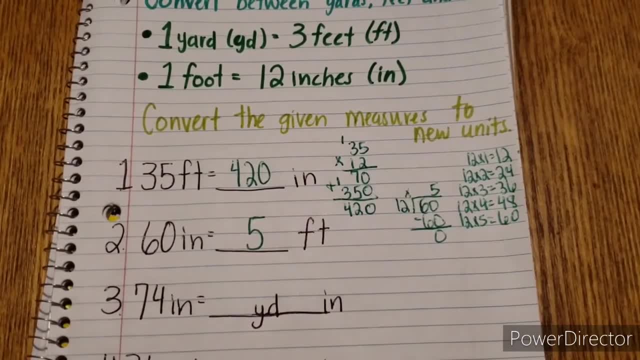 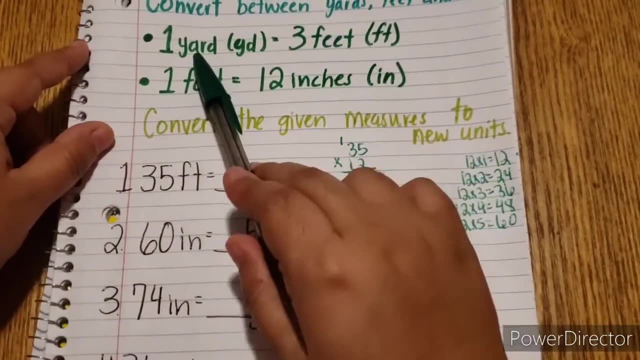 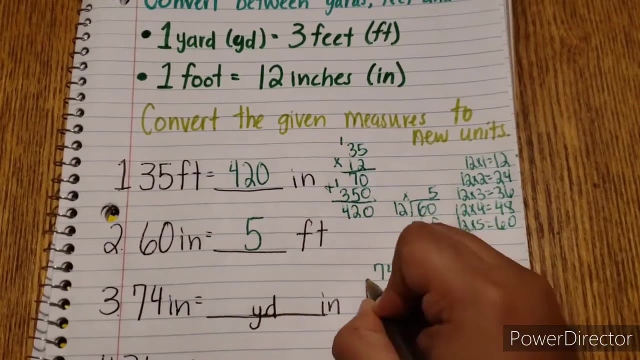 So let's see why it says yard and inches. Let's work out the problem. So what we need to go to is from inches to feet, right here to yards. So the first thing we would do is 74.. Let's go to the next one: 74 divided by 12, so 12 times what equals 74.. 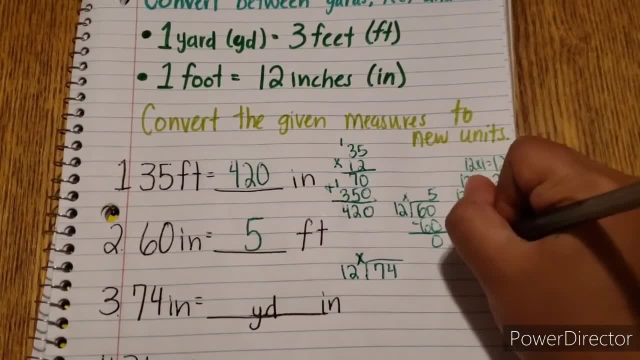 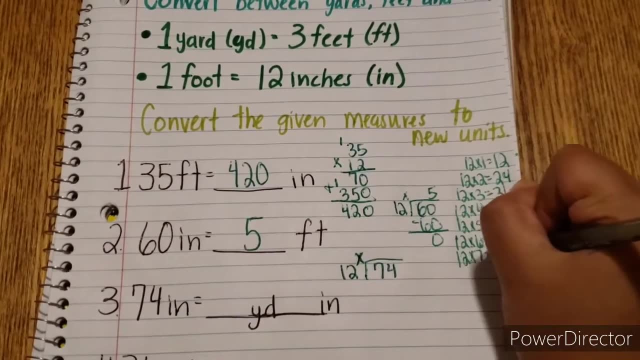 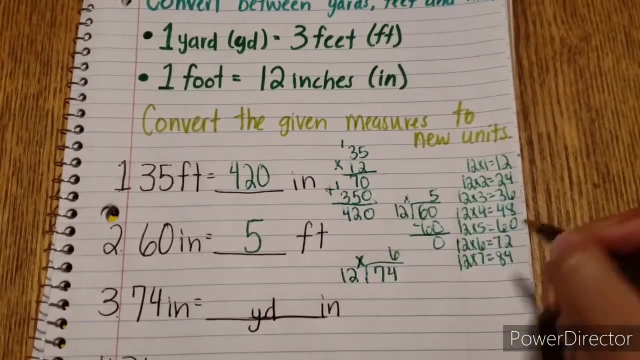 So let's continue this. So we have: 12 times 6 equals 72,, 12 times 7 equals 84. So the closest is 72. So that is 6. So 12 times 6 equals 72. We subtract that and that is 2.. 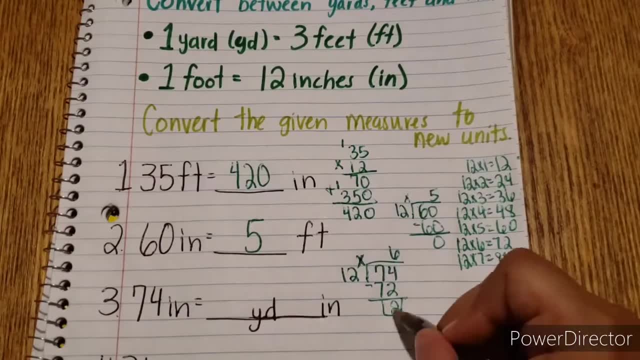 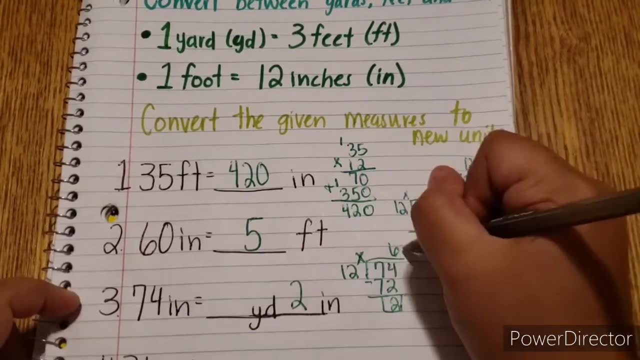 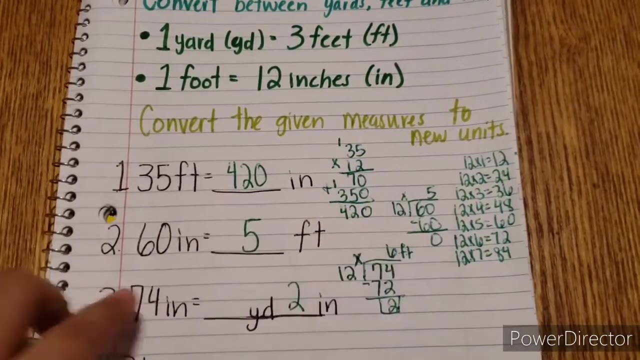 So that is the remainder. So that is the 2 inches. So now let's see how many yards we have. So here we have 6 feet. Now, remember, we have to go from feet to yards. So what we would do is 6 divided by 3.. 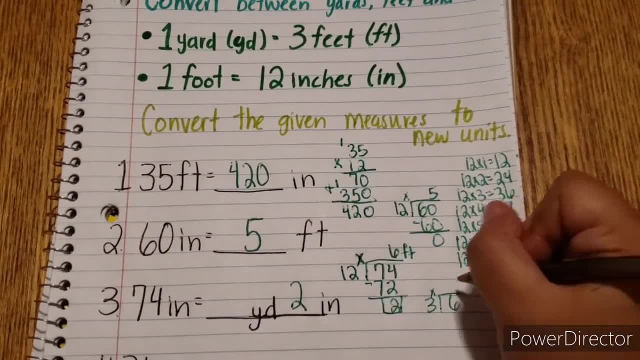 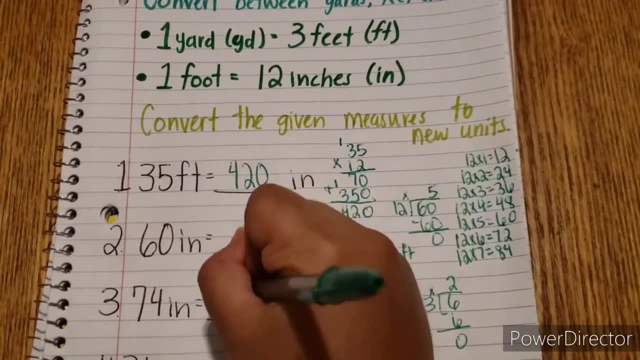 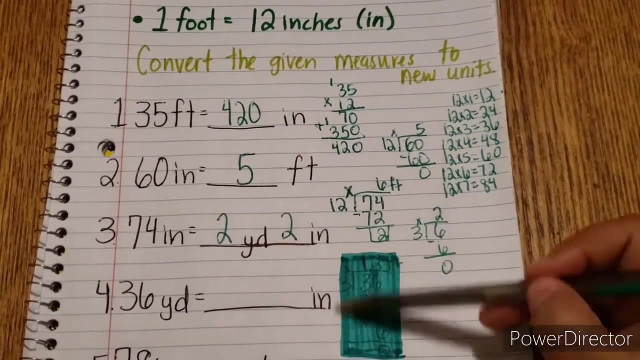 Three times what equals 6?? That is 2.. Three times 2 equals 6.. Minus 6 is 0.. So the answer is 2 yards and 2 inches. So let's get started with number 4.. I started it but I made a mistake, so I went ahead and covered up that mistake. 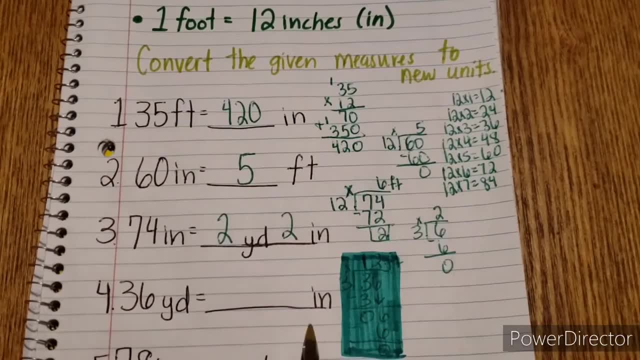 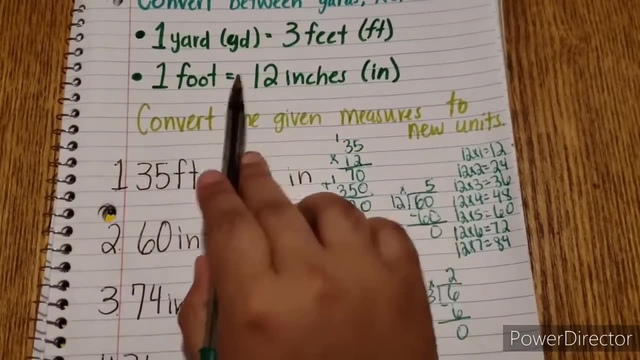 So let's go into it. So here we have 36 yards and we want to go into inches, So in 1 yard there is 3 feet. We want to go from yard to feet, to inches, So we have 36 yards. 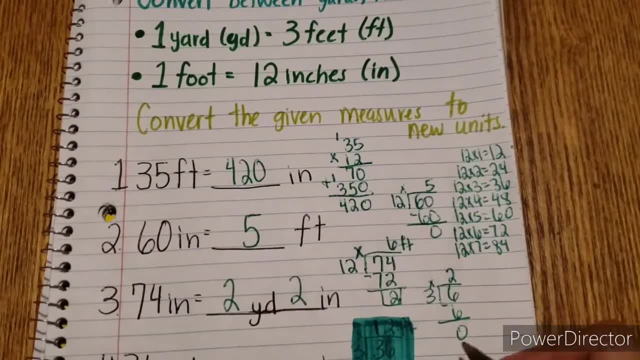 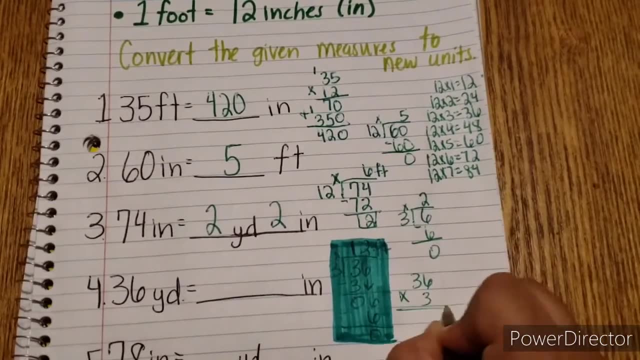 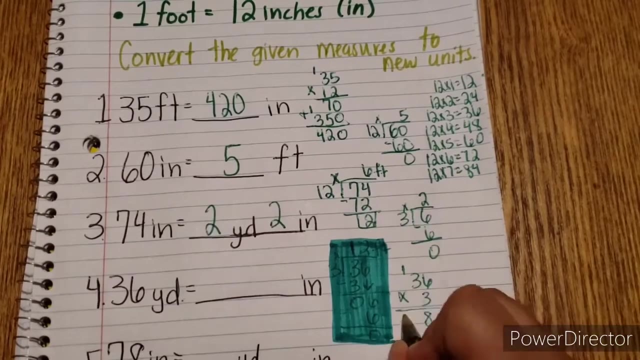 36 yards. how many feet are there? So 30,. what we would do is 36 times 3.. So let's do that right here. What is 6 times 3?? That is 18.. Three times 3 is 9 plus 1.. 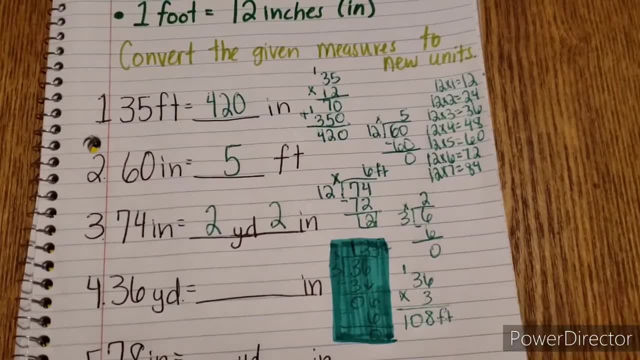 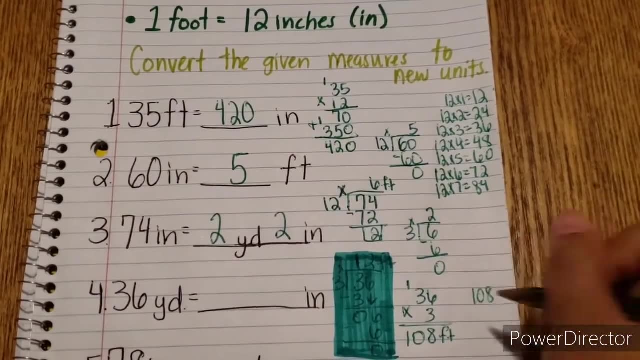 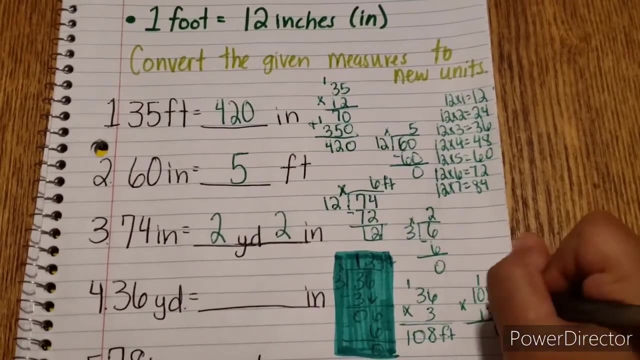 That is 10.. So here we have 108 feet. So now we want to go from feet to inches. So what we would do is 108 times 20.. Okay, So we have 1 times 8. That is 12.. 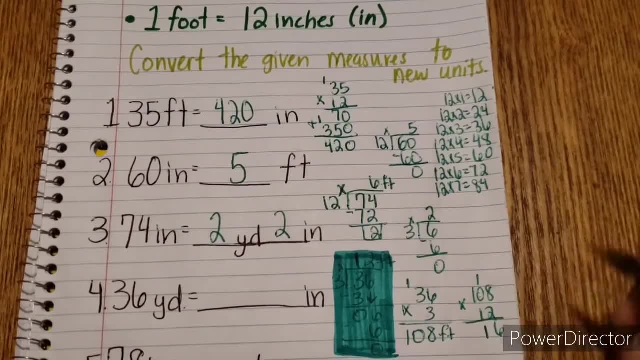 2 times 8.. That is 16.. 2 times 0.. That is 0.. But plus 1 is 1.. 2 times 1 is 2.. We have 0.. 1 times 8.. That is 8.. 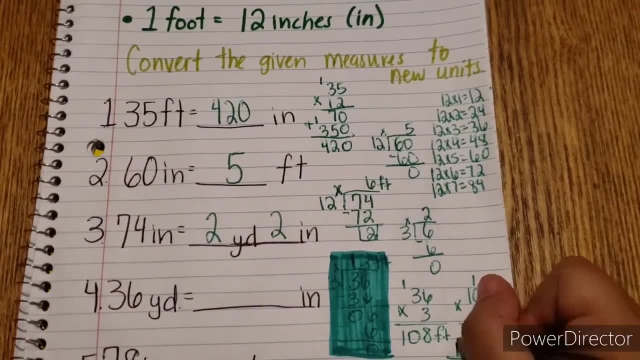 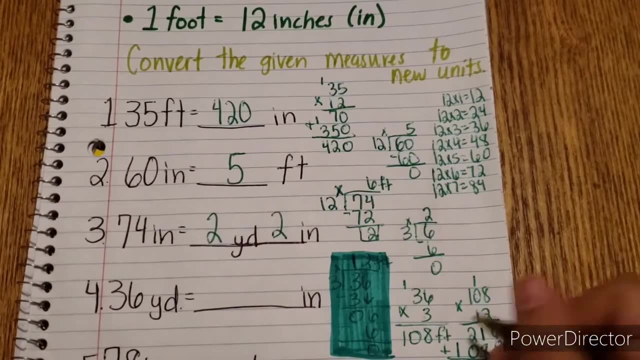 1 times 0 is 0.. And 1 times 1 is 1.. So here we have: 6 plus 0 is 6.. 8 plus 1 is 9.. 2 plus 0 is 2. And 1 plus 0 it is 1.. 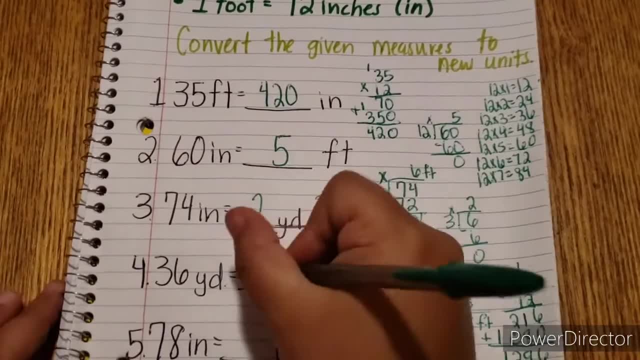 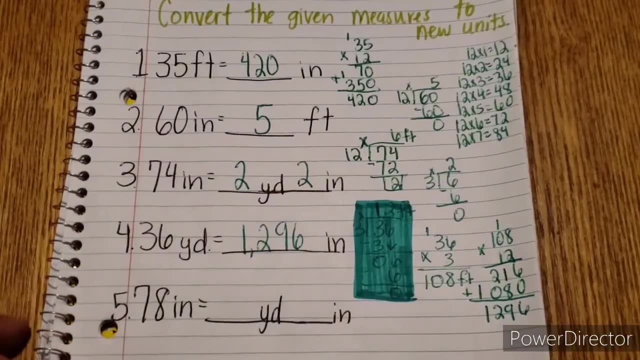 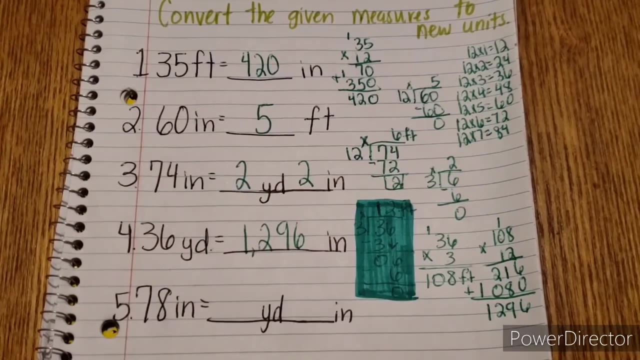 So the answer would be 1,296 inches. So now let's go into number 5.. So right here we want to go from inches to yards, But we will also have some inches left over. So let's work it out to see what the outcome will be.